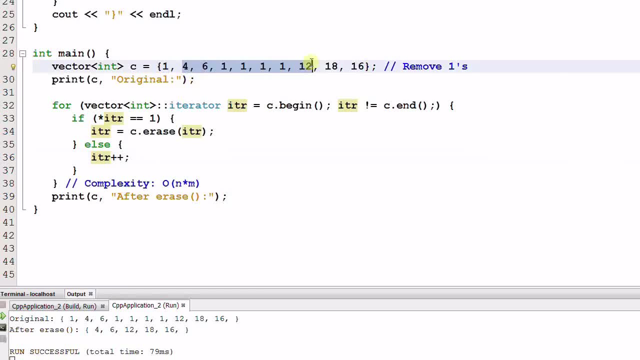 When I remove the first one, all the items after that are moved one item towards the front, And when I removed the second one, all the items after that are once again moved one item towards the front. This is a very inefficient way of of removing items. If the size of the vector c is n and the number of items to be removed is m, 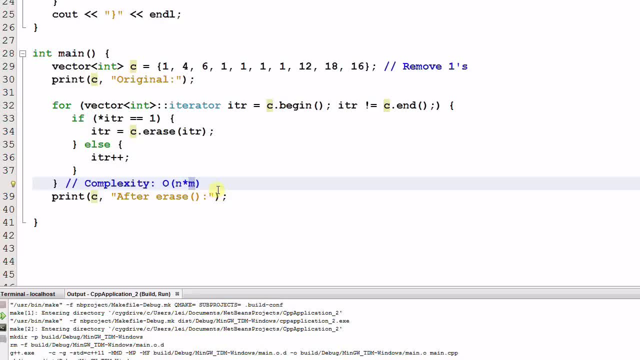 then the complexity of this code is n times of m. This is a very inefficient way of removing items from a vector. A more efficient way is actually using algorithm function remove. The algorithm function remove only moves the unremoved items to the front once instead. 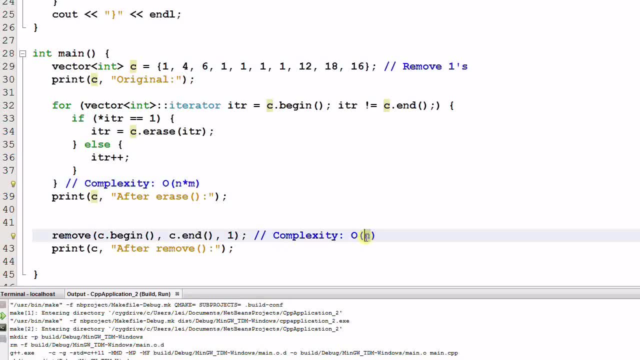 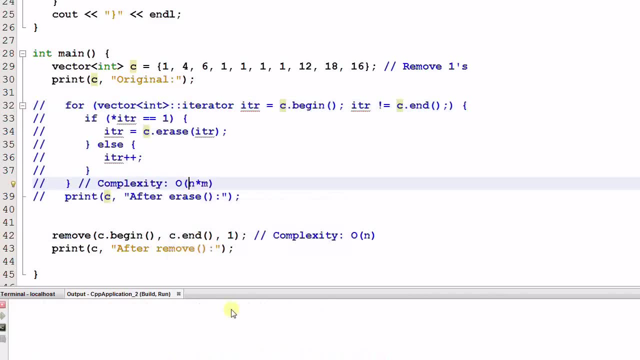 of m times, so the complexity is n. Now let's comment out this portion of the code and see how it runs. Oops, we have a problem here. Although the unremoved items are moved toward the front, as we expected, the vector c: 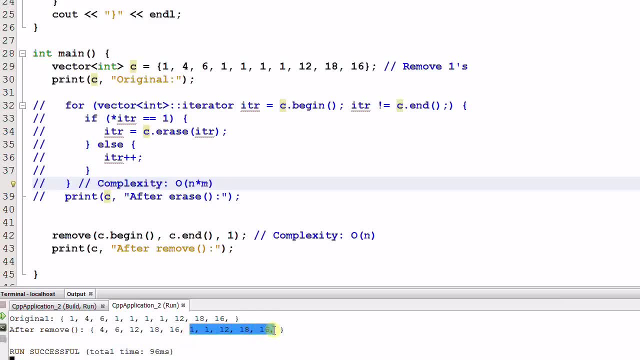 also contains some other items. As I mentioned before, algorithm functions have no idea about the containers. They only know the data through the iterators. So the algorithm function remove has no idea whether the data is stored on a dynamic array or a binary tree or a hash. 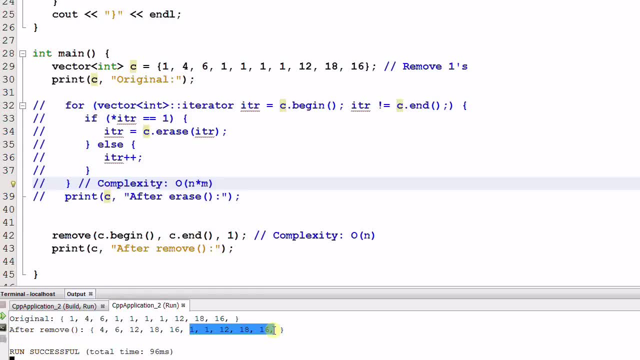 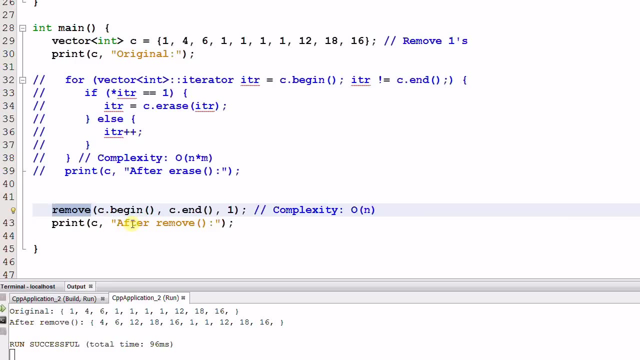 table. That is why it is impossible for the algorithm function remove to actually remove items from a concrete container. So this function remove will do what it can do, which is move all the unremoved items to the front of the vector and then return a iterator which points to the new logical. 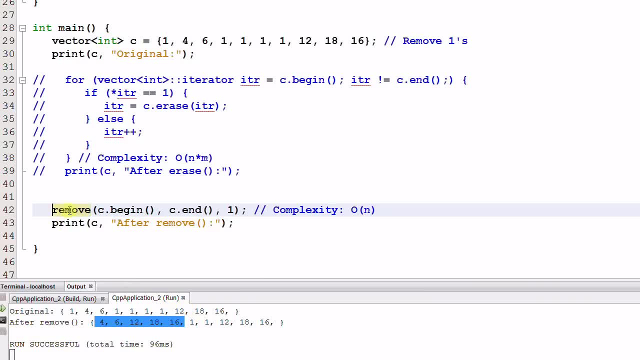 end of the new vector. So to completely the task of removal, we need a pointer iterator to save the new end and then call the rescue function. There used to be a pattern critical to this one, so vibrations added a new request to the new turnaround. 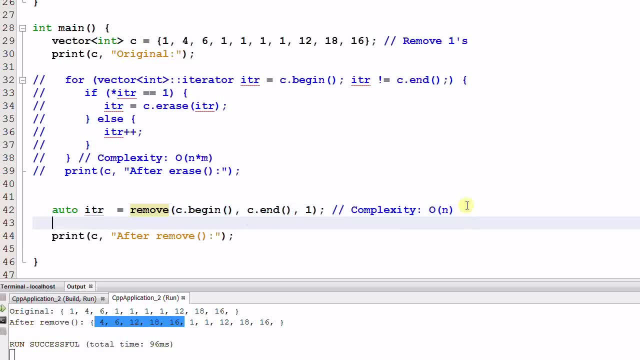 and then call the member function of the vector erase to actually remove the item. Now. let's run it. Now the removal work is truly finished. We have removed all the ones in vector C. and what will be the capacity of C? Let's check it out. 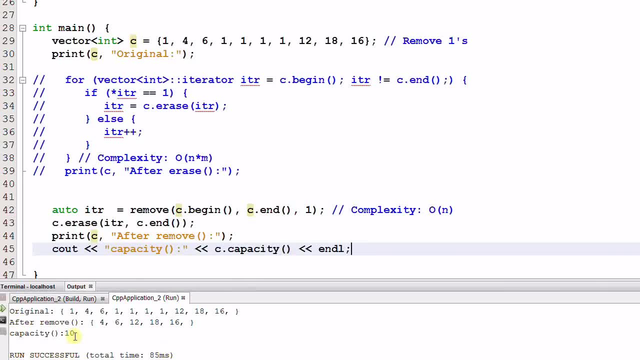 As you see, the capacity of C is still 10.. We have reduced the size of C from 10 to 5, and C is still occupying as much memory as it does before. If that piece of memory is important to you and you want to release them back to the system, there's one extra step to do. 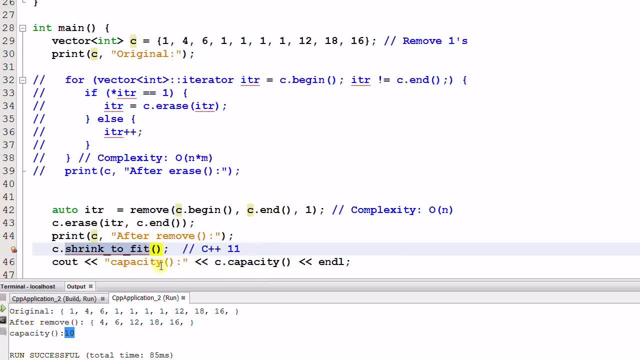 You can call the function shrinkToFace, Which will release the unused memory back to the system. Now let's run it. Now. the capacity of C is reduced to 5.. However, this function, shrinkToFit, only exists in C++11.. If you are using old C++, you can use the swap trick. 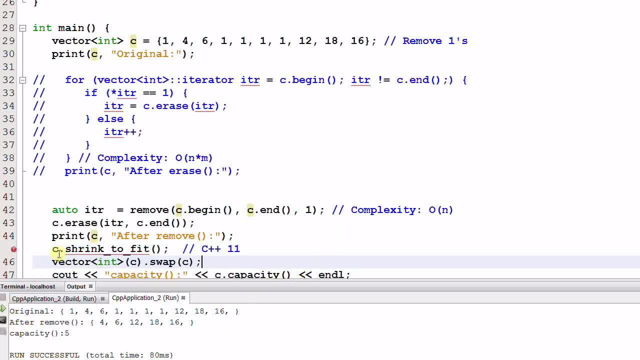 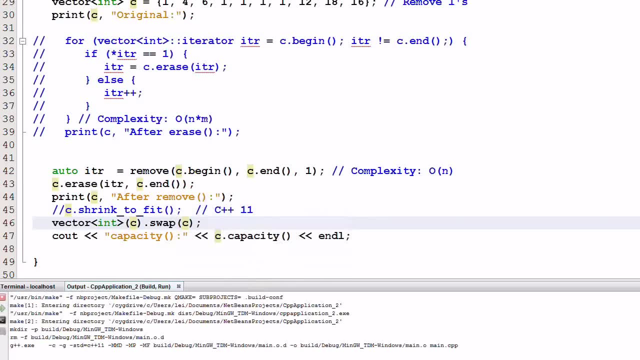 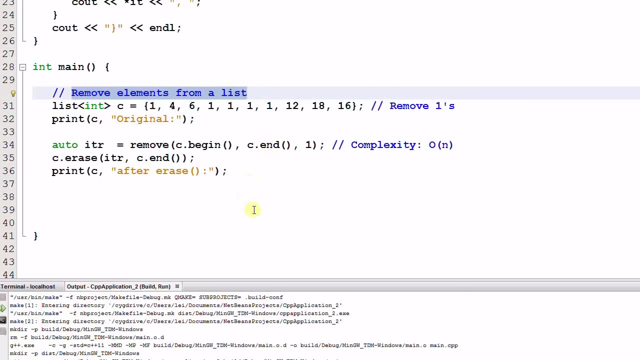 And this should also do the job of shrinking the memory. Now let's run it. As you see, now the capacity is 5, so the memory is shrinked. Now let's talk about remove elements from a list, Since we've just learned a lesson from the vectors, example. 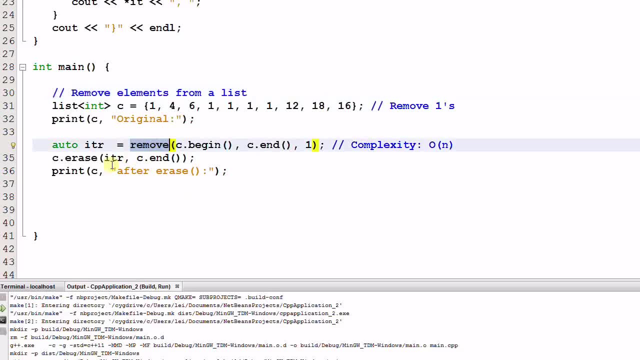 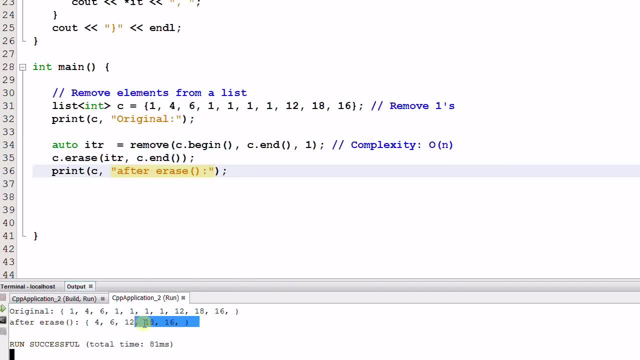 we'll use the algorithm function remove, Followed by the member function erase And run it. This also gets the job done for a list, but this is not the optimal way of removing items. List has a member function called remove And this remove function can do the job of removing items more efficiently. 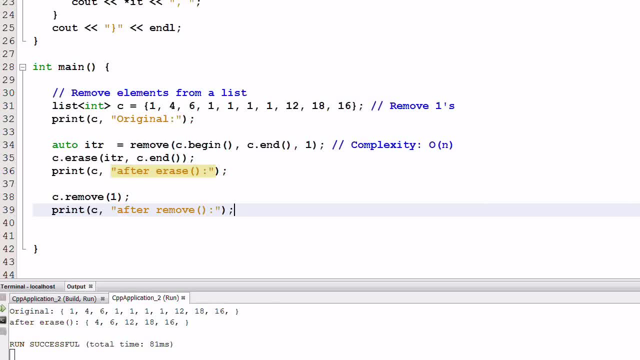 Why is that? As we mentioned, the algorithm function remove does the job by moving the unremoved items toward the front of the vector, But the member function remove doesn't do that. The member function remove knows the data structure of a linked list. 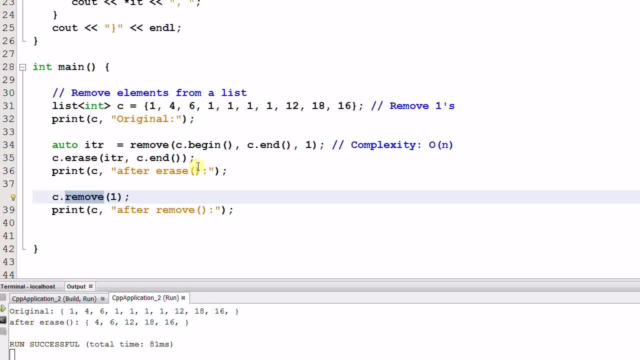 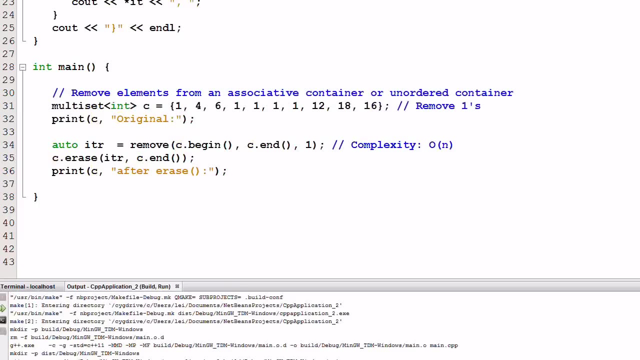 so it does the remove by tweaking the forward pointer and the backward pointers, which is more efficient. So now, this is a fast way of removing items. It's a faster, easier and cleaner way of removing items for a list. Now let's look at remove elements from an associative container or unordered container. 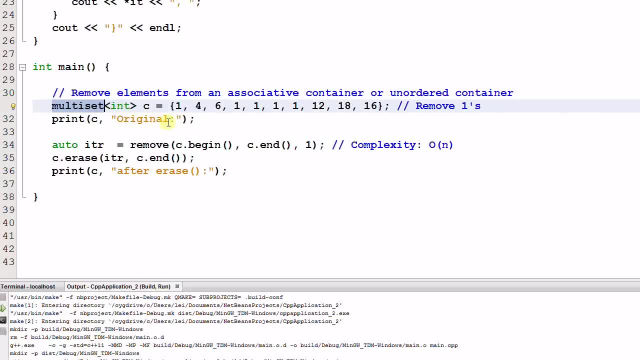 We have a multi-set of integer c and we want to remove all the ones. We look at the multi-set member function and we don't see a dedicated remove function like the list does. So maybe we should go back to use the remove algorithm, followed by erase function. 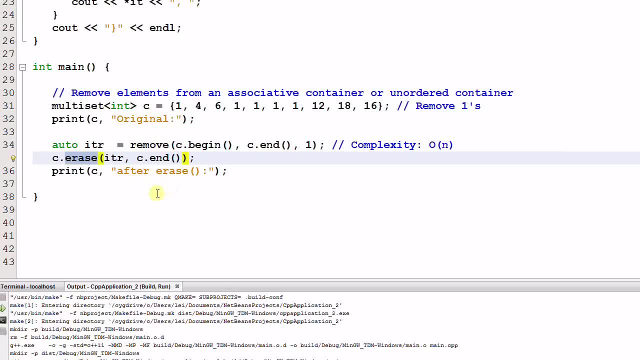 The answer is no, you don't. Although multi-set doesn't have a dedicated remove member function, it has a much better version of erase function. The multi-set's erase function can remove items by value and do it quickly. Let's comment out this portion of the code and run it. 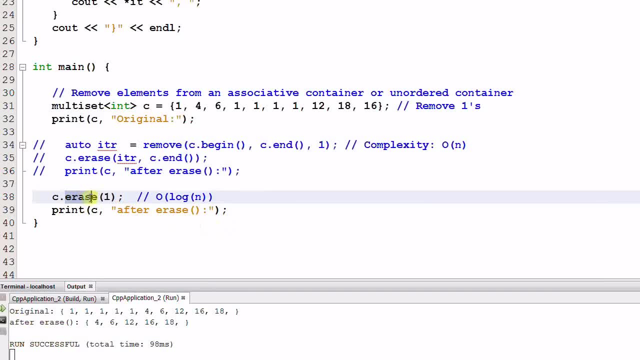 The multi-set's erase function only needs logarithmic time to do the removal instead of linear time, And for unordered container it is even faster. It only needs amortized constant time to do the erase. So in both case you should use the member function erase. 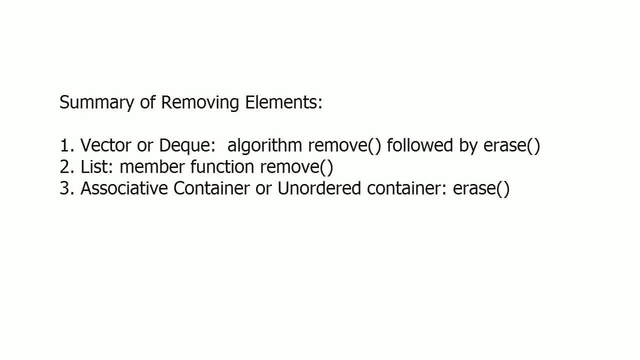 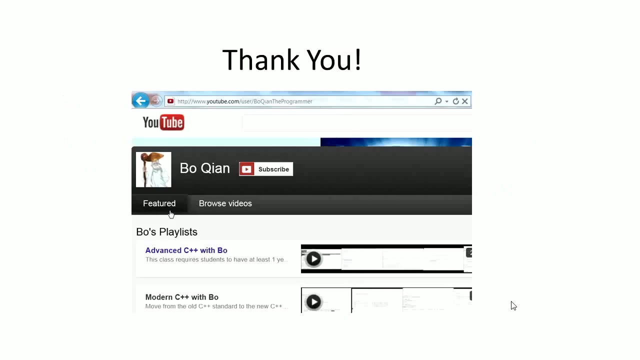 to do the function of removal. A summary of removing elements from a container: For vector or deck: use algorithm remove, followed by member function erase. For list: use member function remove. For associative container or unordered container: use member function erase. That's all for today. 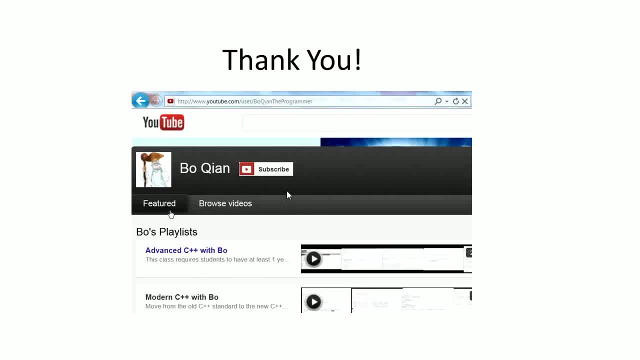 Thank you for watching. Feel free to subscribe to my channel so when I post a new video you will be updated, Or you can go to my channel's homepage and see what I am offering today. Bye, bye.